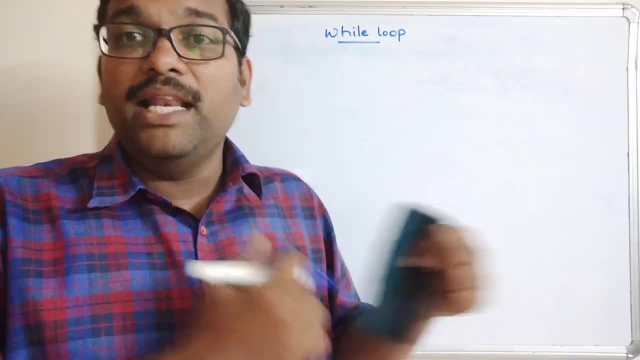 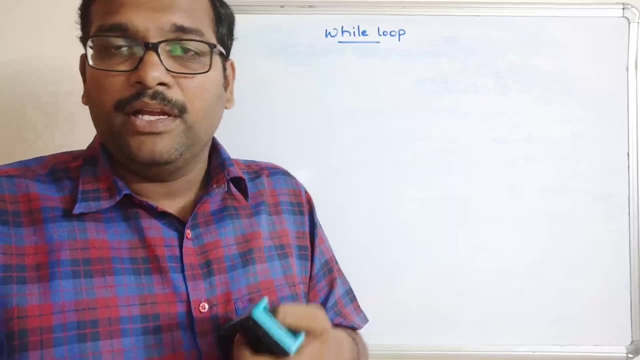 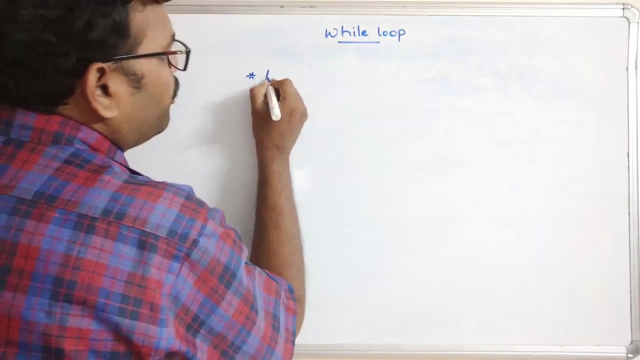 if that doesn't happen, the complete process may lead to infinite loop. That means always the same set of instructions will be executed repeatedly. So for the implementation of this while loop or for loop, the three things should be focused. The first one, loop variable. 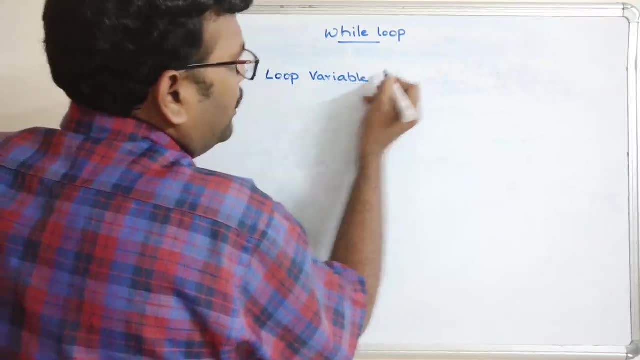 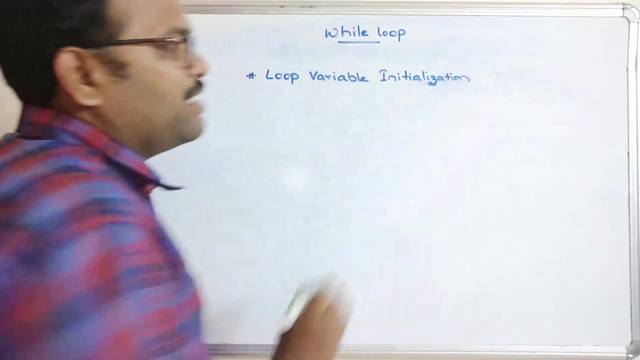 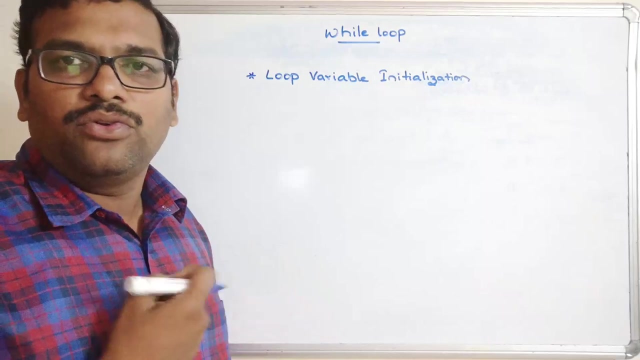 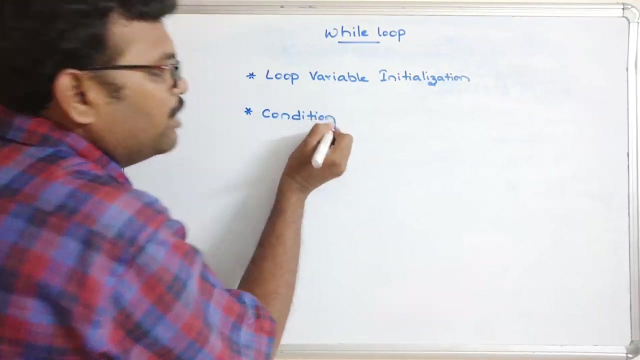 initialization. Loop variable initialization. So loop variable initialization. so we need to initialize a loop variable. okay, to perform in the iterations. so that means assigning an initial value to the variable. and then we need to focus on condition. so we should write the condition very carefully, because this condition is mainly used to terminate the loop. okay to stop. 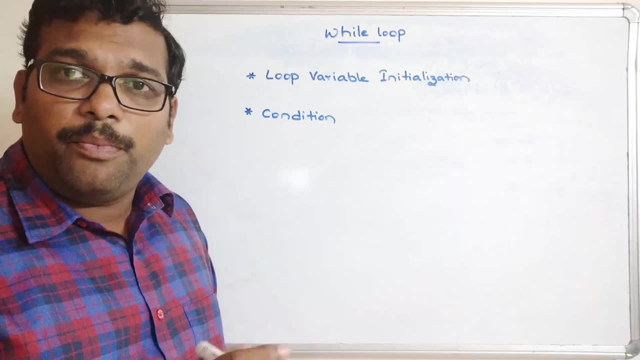 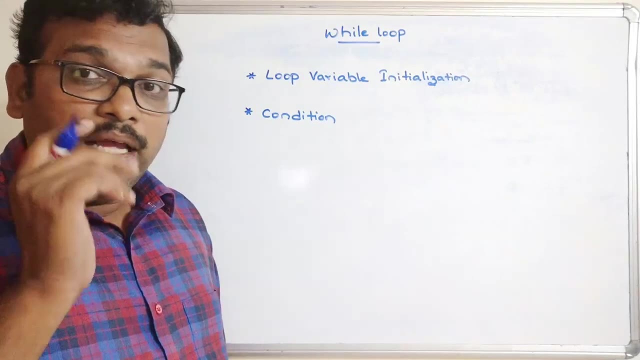 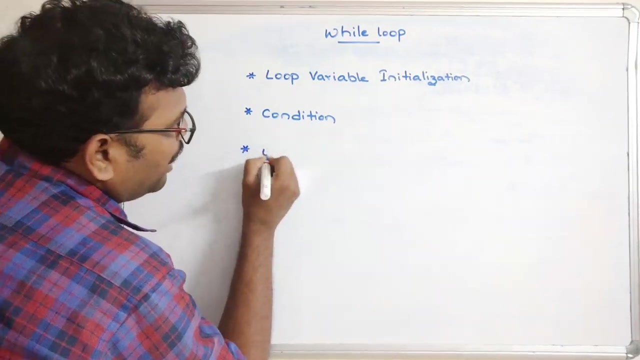 the iterations. so if the condition is not written properly, the instructions will be keep on executed. that means it may lead to the infinite loop, so the instructions will be get executed until this condition becomes false. and the third one: updation. so the third one is updation of. 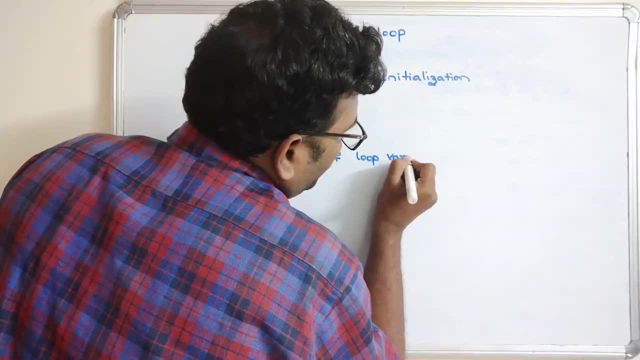 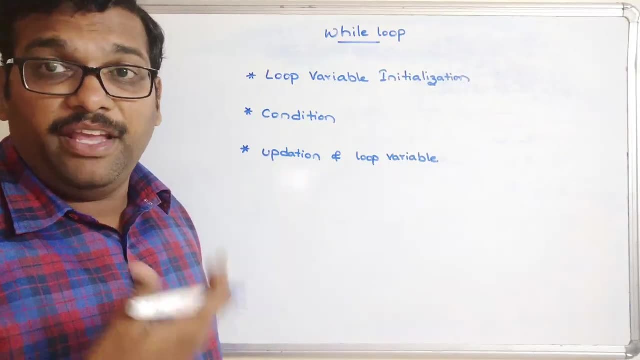 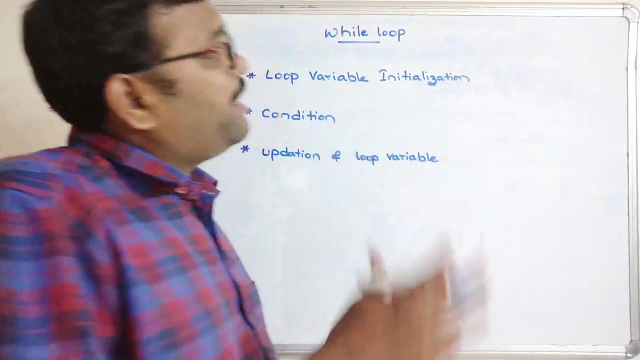 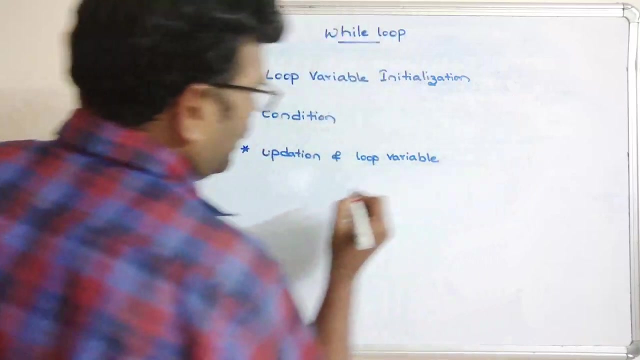 loop variable- updation of loop variable. so after every iteration, this loop variable should be updated. it may be incremented or an incremented, but that updation should be done, okay, so for both iterative statements for loop or while loop, we have to follow the same thing, and this is also called as entry controlled loop. entry controlled loop. 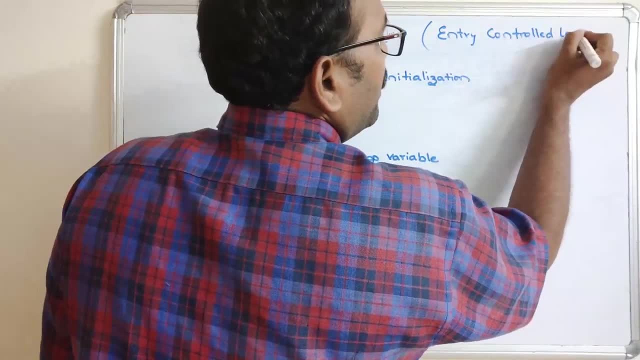 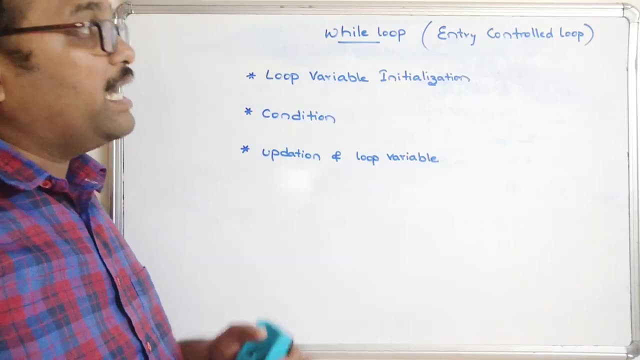 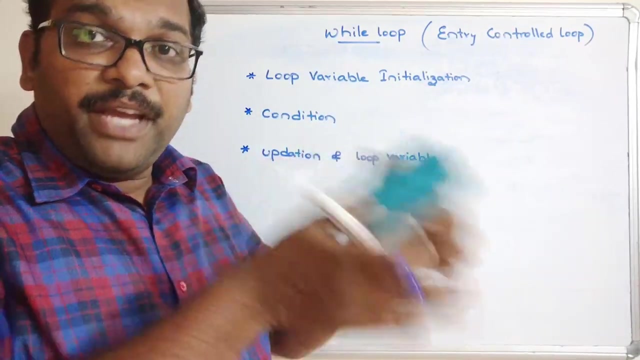 because before entering into the body, before the ordering, then the control goes to the instructions of the while loop. the condition will be verified and if the condition is true, then only the control will enter into the loop. so at the beginning itself we are checking the condition. so that's why we call it as an entry control loop. so the syntax. 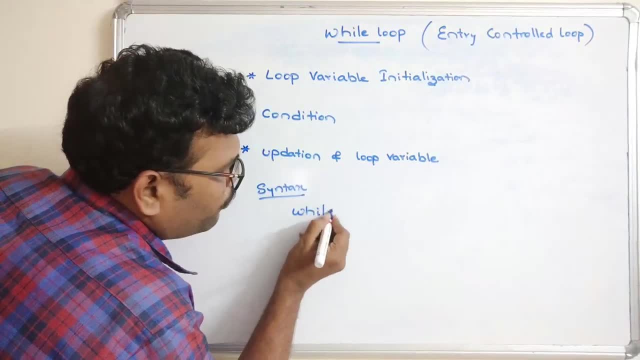 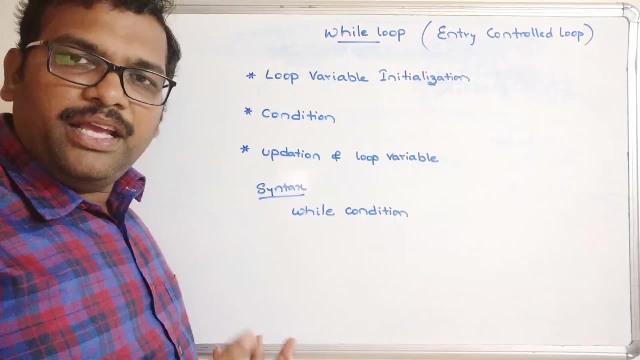 for a while loop is we have to use a keyword called while and followed by the condition, and we need to write a condition, and this condition can be assumed. so for the a simple condition or a compound condition. so if it is a simple condition, we are going to use the. 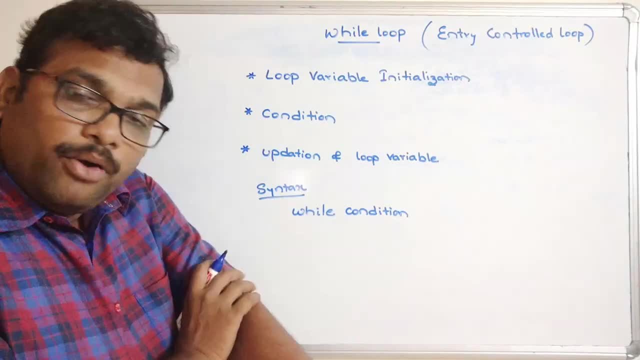 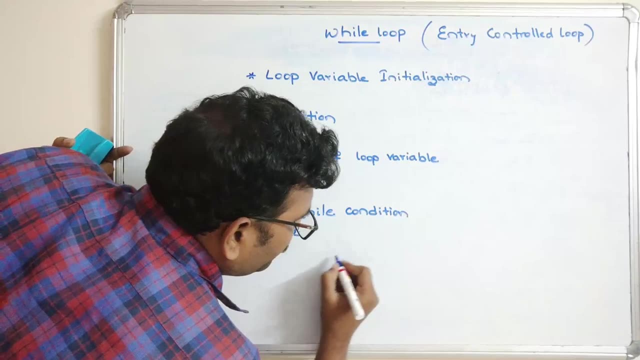 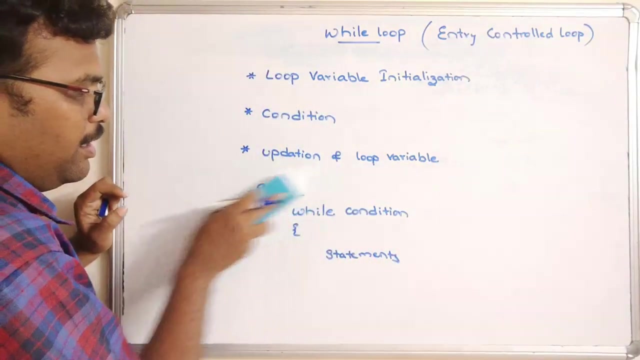 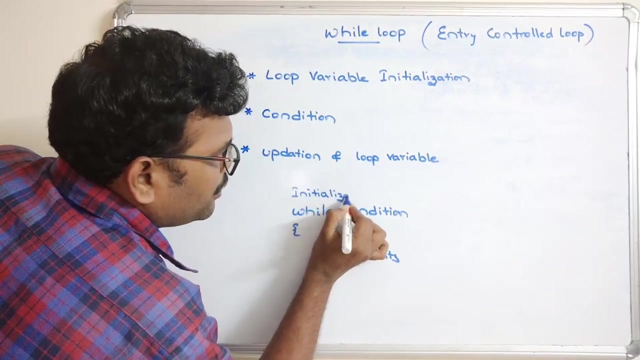 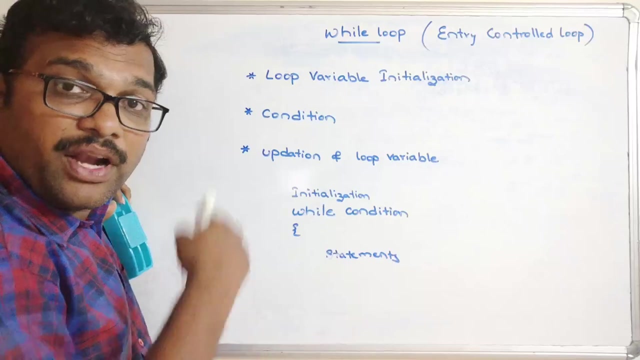 relational operators and if it is a compound condition we have, we are going to use some logical operators- right and curly braces- and here you need to write the statements. you need to write the statements and here we need to give the initialization. initialization. so if you write this initialization inside the while loop, so for every iteration the 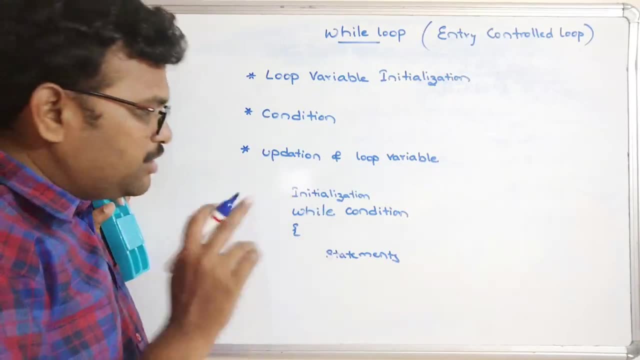 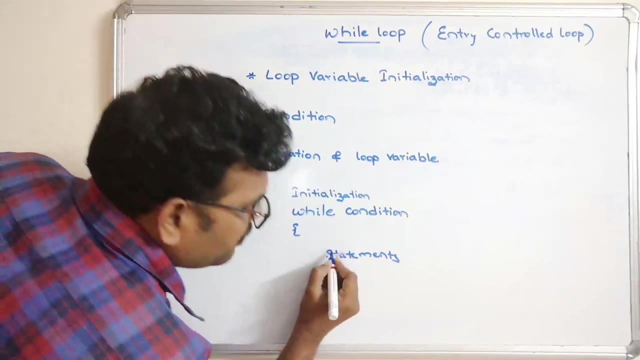 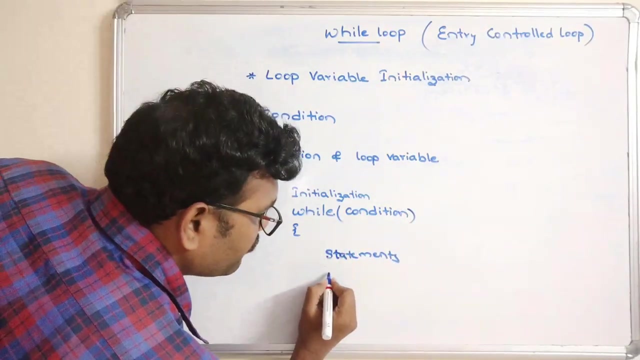 value will be initialized to same initial value, right? so initialization should be done above the while loop. so before the before control entering into the while loop, and after that we have to write down the while condition and statements, and after that we need to write the updation. 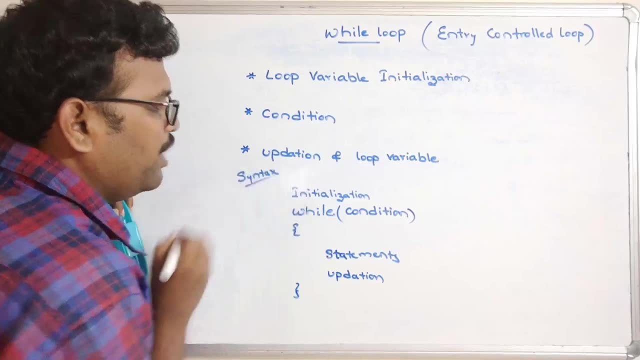 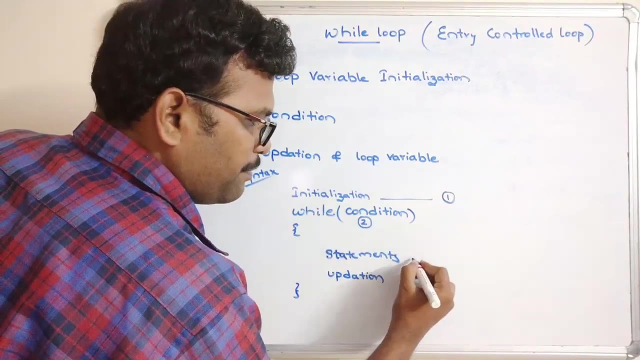 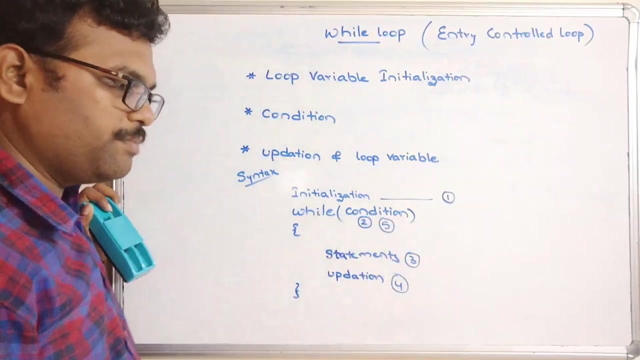 so this is the syntax of while, and the first step is this one and second step is a condition, and the third step statements. and a fourth step, updation. and a fifth step is condition. again, it will check the condition. okay, after completion of this closure brace, it will again check the condition and if the condition is true, 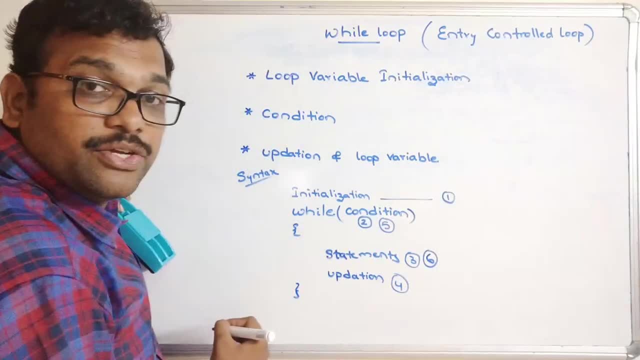 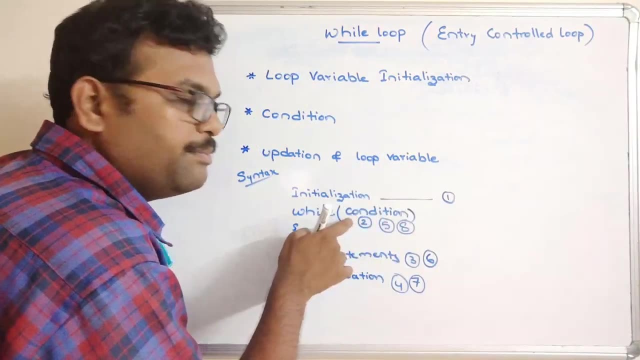 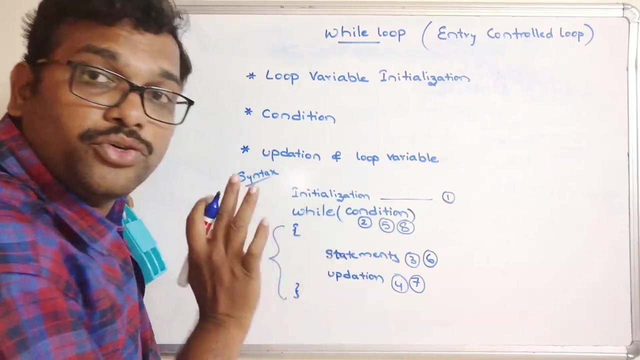 again. the sixth one will be: statements were being executed, and after that seven and again 8 will be the condition. So this will be repeated until this condition becomes false. So the control will enter into this particular loop only when the condition becomes true and when the condition 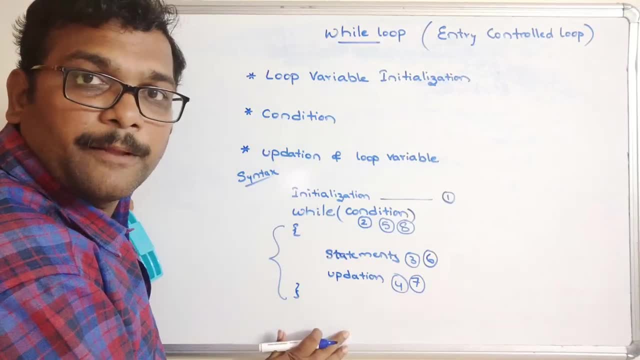 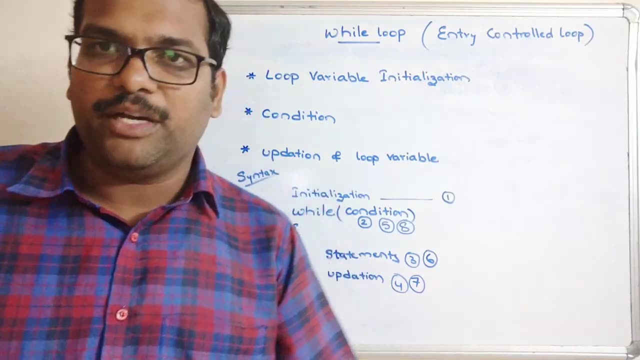 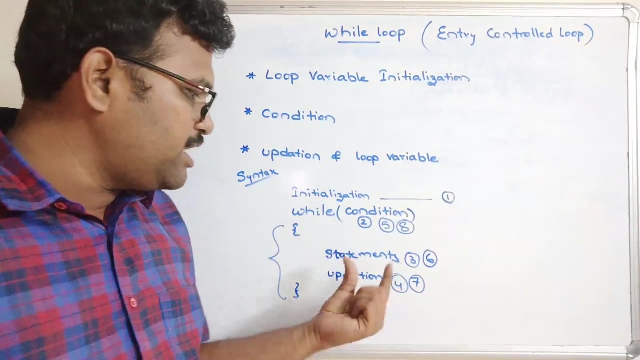 becomes false, the control will lever into this loop. So this is called a while loop and this is a one of the control structure which we call it as an iterative statements. So every time the statements are being executed is called as an iteration. So one time, one time the statements 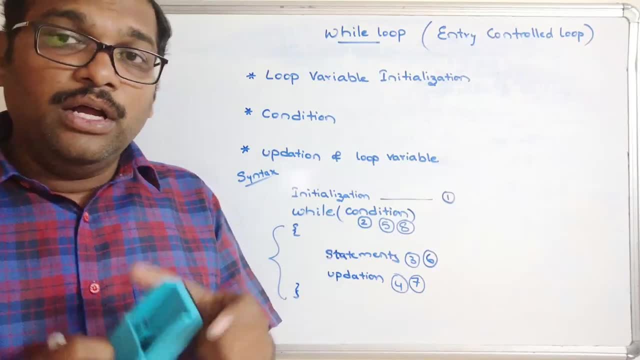 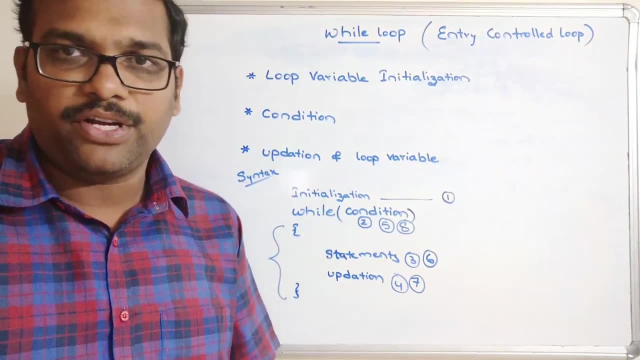 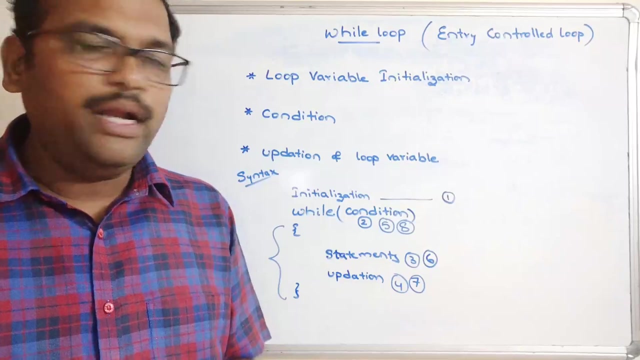 are being executed is called iteration. So if these statements are executed five times, we call it as a five iterations. five iterations So that we have already discussed in our previous session. that means the explanation of for for loop, right? So hope you understood this while loop and now. 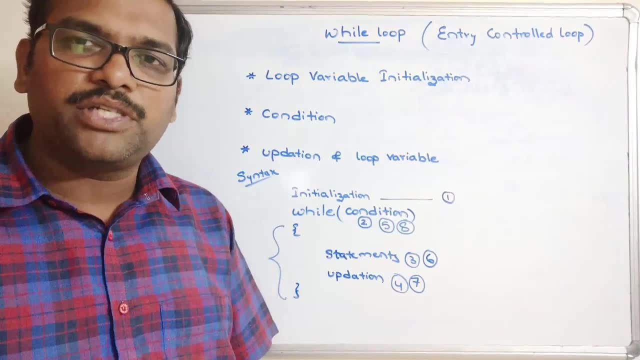 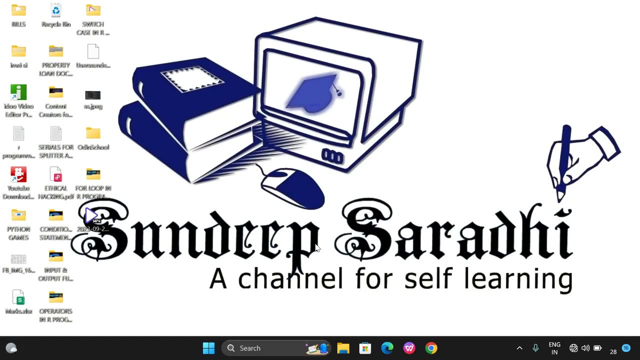 let us move on to the system. I will show the demonstration of this particular while loop in RStudio. So let us move on to the system. Hello friends. so just now we have seen the complete syntax of a while loop. Now we'll see the 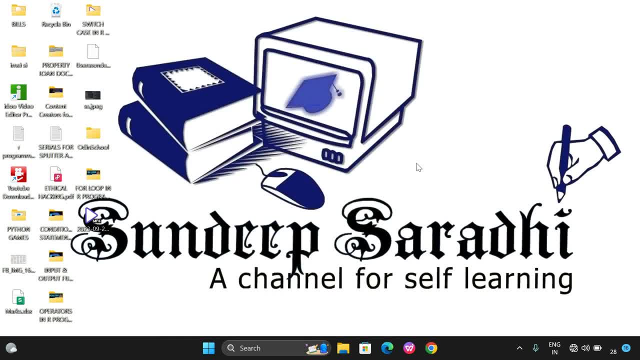 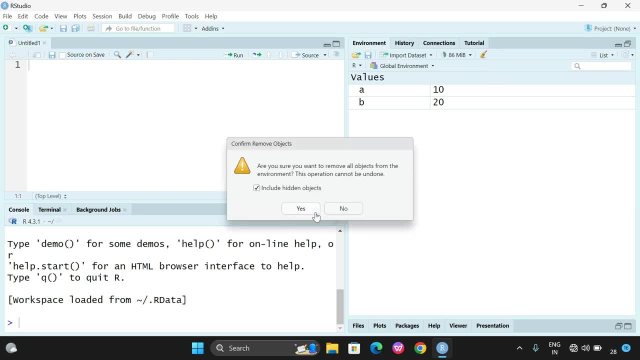 implementation part. So let us open the RStudio and then we'll remove the complete existing data and then we will start. So let us take the initialization of the loop variable. I will take the loop variable as i and i'll initialize to 0. And now I'll write the while loop. 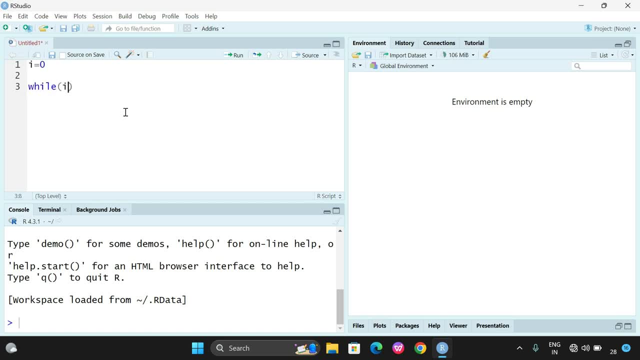 while, and now I have to write the condition- will write the condition as I less than 5. that means whenever I becomes less than 5, then immediately the control will enter into the loop. so whenever this condition becomes false, then that means whenever I becomes the value of I becomes greater than 5. 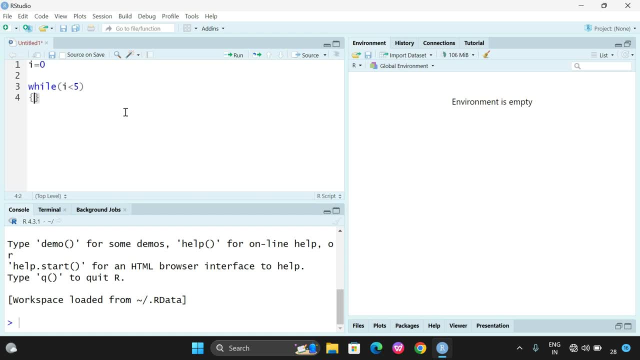 immediately the control will exit from them, right? so here I am giving the body of the loop, so I will give print I and I need to update the variable every time. I need to update the variable because if you are not updating the variable, it may lead to the continuous execution. that means the infinite loop. because I value 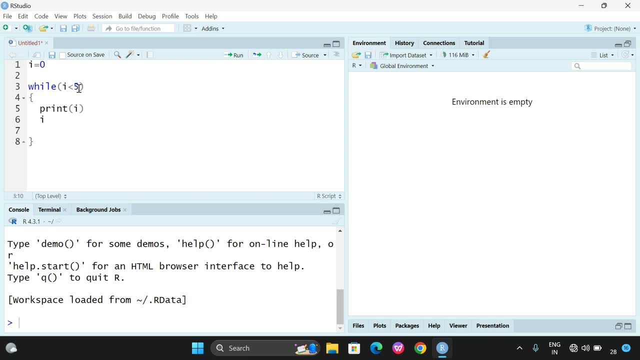 will be 0 initially, so 0 less than 5 it is a true, so this statement will be executed. and if you are not updating the loop variable automatically for every time, every time 0 is less than 5, that means every time the condition becomes true. only then it may lead to the infinite. 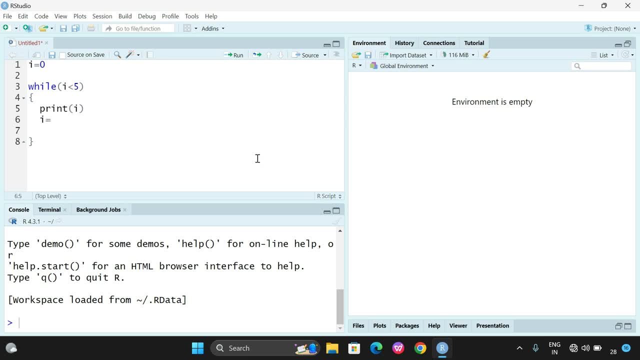 loop right, there is no termination. so here I need to update the variable. so I am updating the variable with the 1. so after one iteration I becomes 1, after second iteration I becomes 2, after third iteration I becomes 3. so every time we are checking the condition with the change updated variable. so at one. 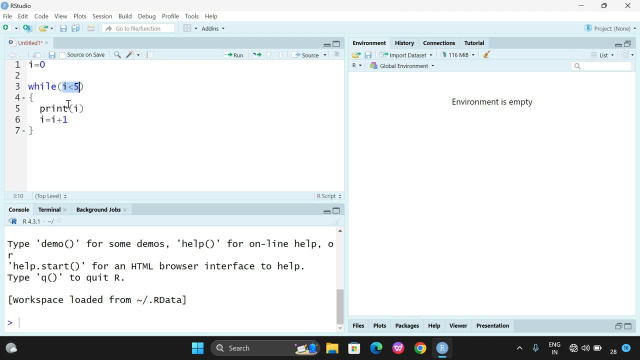 particular time, the I value will be automatically greater than or equal to 5, so at that time the variable will be updated and the condition will change automatically: greater than or equal to 5, so at that time the condition will be position, so the loop will be terminated. right? so this is a simple code to display the complete. 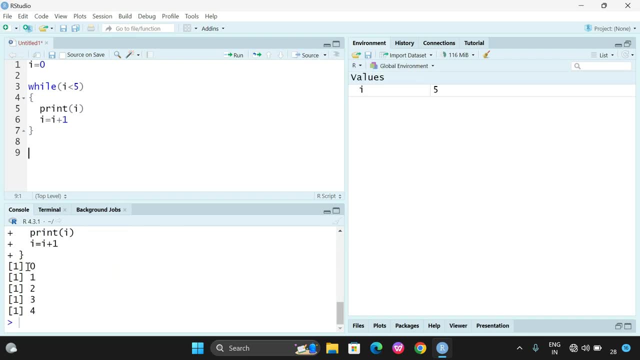 details. so let us execute. source. you can see it will start from 0 to 4.. if you go with a less than or equal to 5, and if you go with a 1, so will. it will display the complete details from 1 to 5. 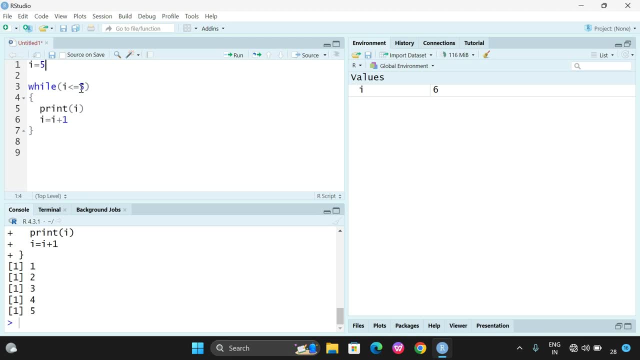 and let us take if it is 10 or if it is a 5 and if it is greater than or equal to 0, right, and here we need to decrease the value. so you can observe, complete details will be repeated. i mean, from first, iteration 5 will be printed and the second iteration 5 will be updated to 4. 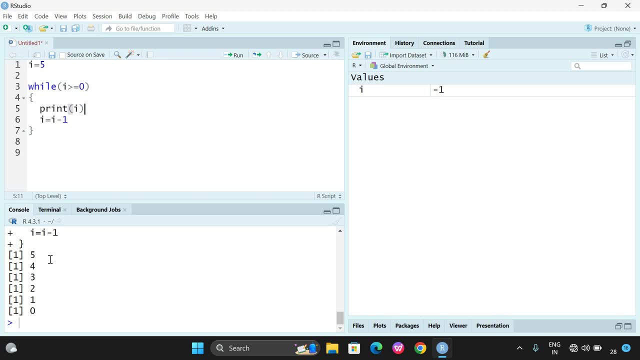 and the 4 will be checked with the condition- and it will be repeatedly- it will be executed. so here, instead of taking this one, we can read one value here. okay, i'll take n is equal to, as dot, integer of read line. enter value of n. right, and here we need to take a loop variable as a 0 and let us take some i greater than or. 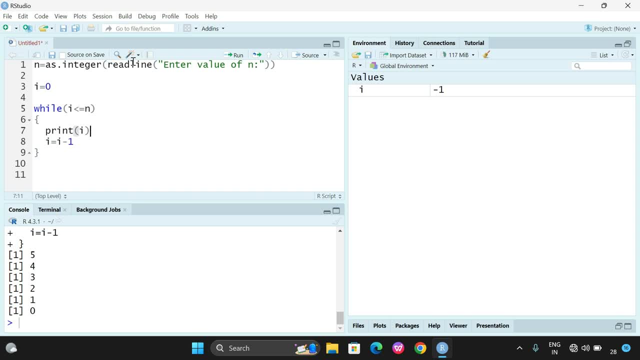 equal to i less than, or equal to n. right, And here you can simply go with this one so that we can prompt. we need to update it, So execute. So we have to enter the value of yen. If I give it as a 10, we'll get the complete values from 0 to 10, because here we have started. 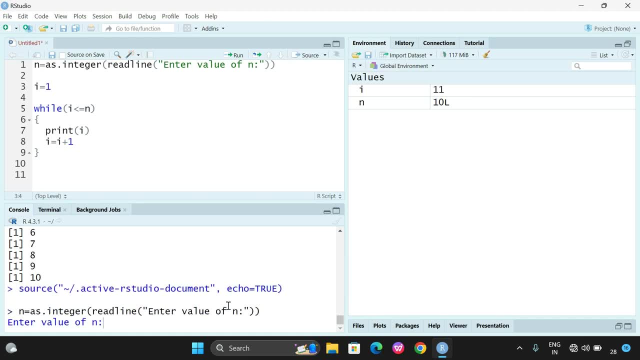 with a 0. So go with a 1.. So simply, you can go with 20.. If you go with the 20, it will display all the values from 1 to 20.. And if you go with the 100, it will display the complete elements from 1 to 100. 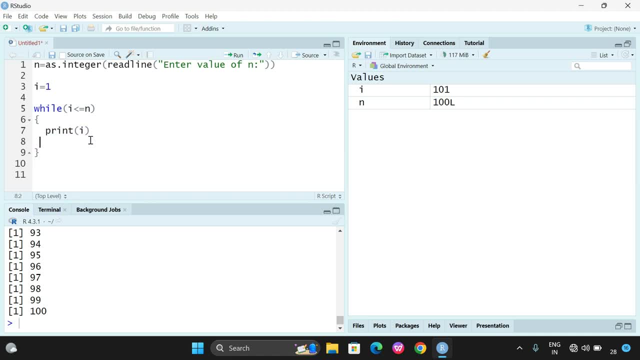 What happens if you are unable to write the updation. So we said that. we said that it may lead to infinite loop. So let us take some 4 and you can see. so it was keep on printing 1 because we are not updating the iValue. 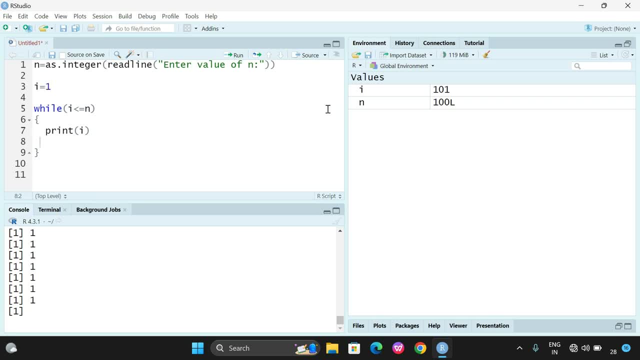 Always iValue will be 1 and always nValue will be 4.. So iValue i less than or equal to yen. that means a 4, right? So simply what happens here. So it will be keep on moving. So there is no updation of the loop variable.